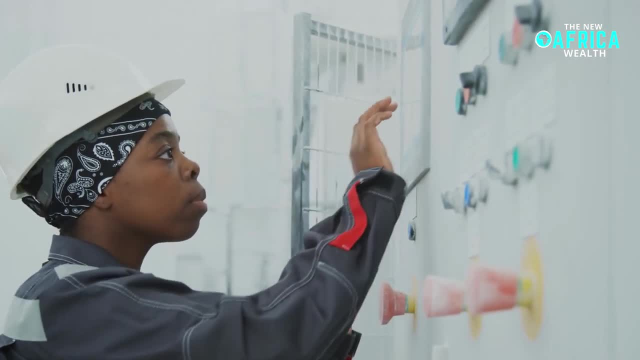 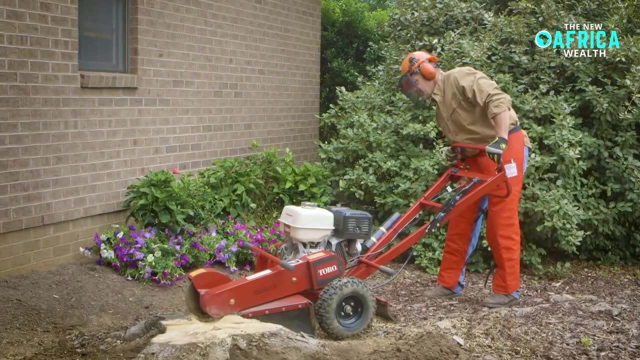 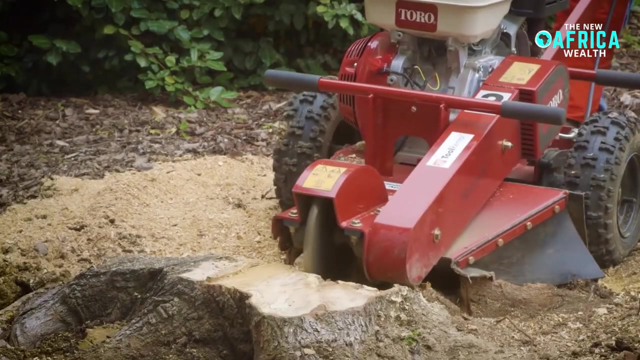 and subscribe to The New Africa Wealth for more content. The tree stump grinder presents a lucrative opportunity for outdoor equipment enthusiasts. As many individuals tackle tree removal on their own, they are often left with stubborn stumps and no means to remove them. Seizing this gap in the 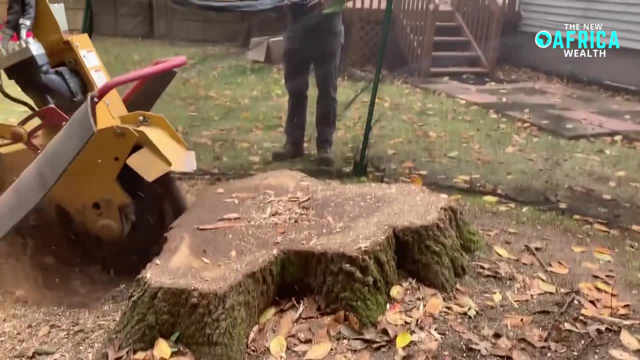 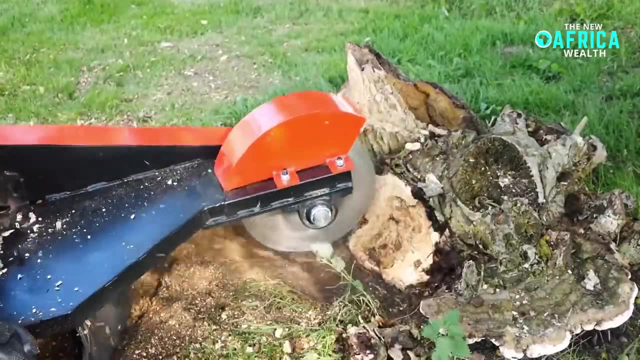 market. you can offer your services to homeowners charging a premium hourly fee due to the relatively quick nature of the task. Additionally, renting out the tree stump grinder when not in use can generate passive income, further boosting your revenue stream With an average nationwide cost. of about $400 in the US for stump removal. investing in a tree stump grinder- which typically costs $2,000 to $3,000, can be a great way to save money, But if you're looking for a tree stump, 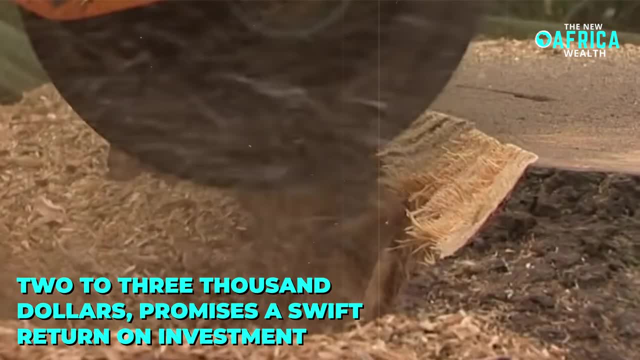 grinder. you can also opt for a tree stump grinder, a tree stump grinder and a tree stump grinder. The tree stump grinder, which costs about $100,000, promises a swift return on investment and opens the doors to a potential side business. While the benefits are promising, some considerations. are essential to ensure a successful venture. Obtaining liability insurance is crucial to safeguard yourself and your business against any unforeseen incidents. Moreover, effective advertising and marketing efforts are necessary to attract clients and establish your presence in the market. Potential earnings could be between $30,000 to $5,000.. A tree stump grinder. can be used to pack a bag of spoons and make these bags as small objects as possible. The tree stump grinder is a tough, bulky and expensive tool that can be used toomblaze or billboard a bunch of speeding birds or to fill rear windows with an even lighter roof. The tree stump grinder. 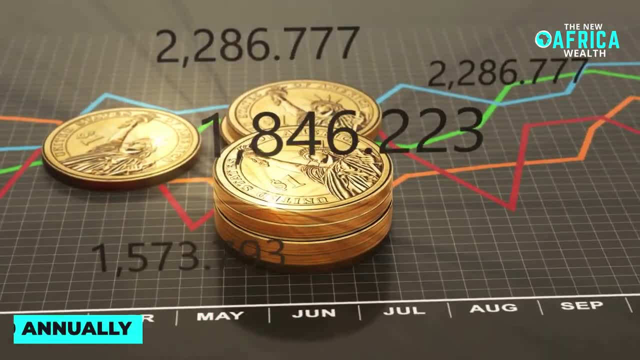 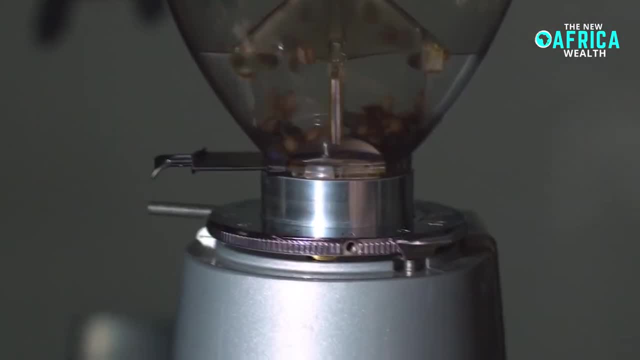 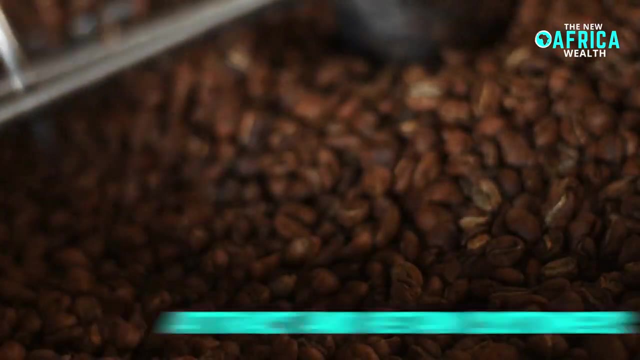 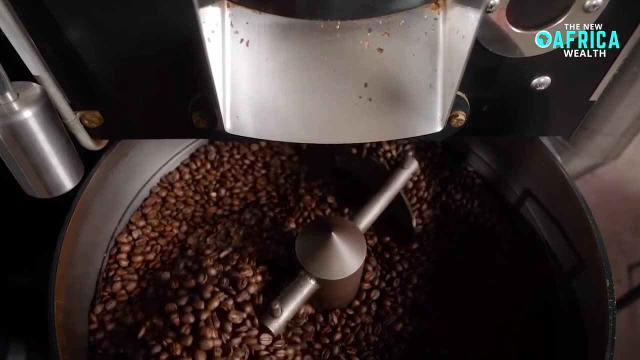 and one hundred thousand dollars annually. Coffee roasting can indeed be a lucrative venture, offering coffee businesses a smart way to attract and retain customers. By roasting their own coffee beans, caftas and coffee shops can create unique flavors, stand out from the competition and establish a strong brand identity. 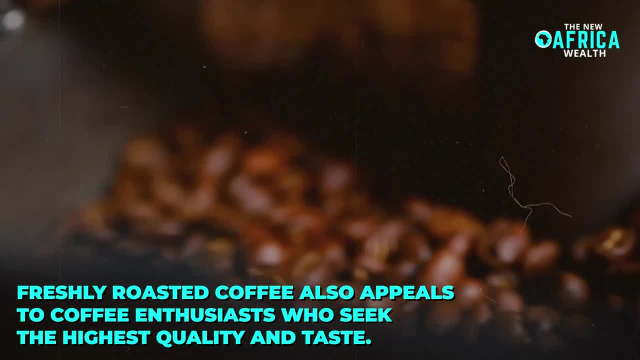 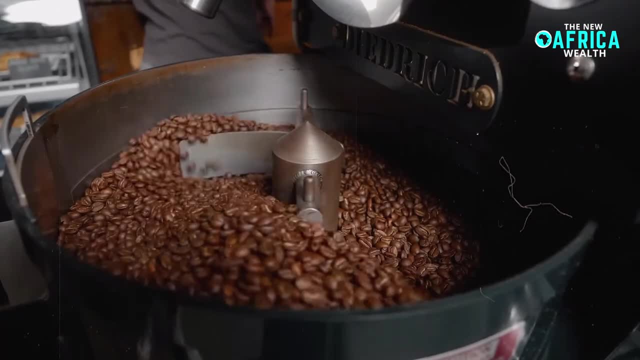 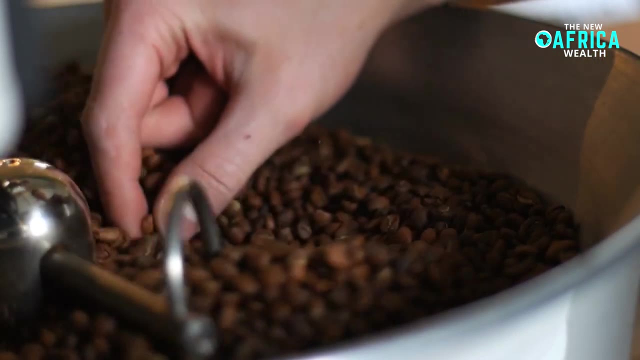 Freshly roasted coffee also appeals to coffee enthusiasts, who seek the highest quality and taste. With the ability to control the roasting process, businesses can fine-tune their coffee profiles, ensuring consistent and exceptional brews that keep customers coming back for more. However, one of the main challenges for entrepreneurs 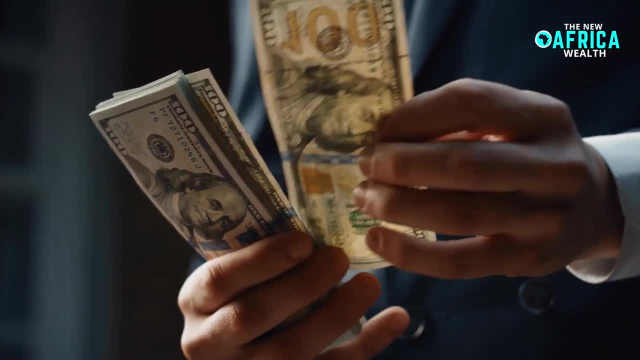 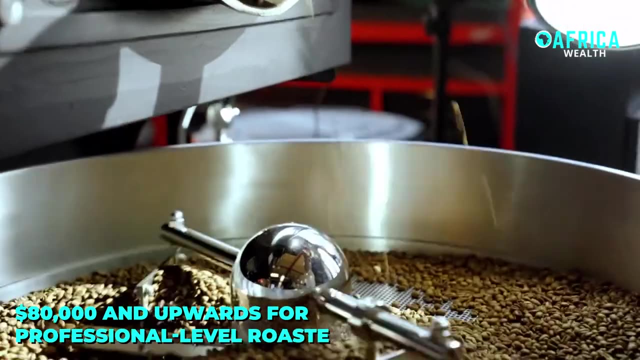 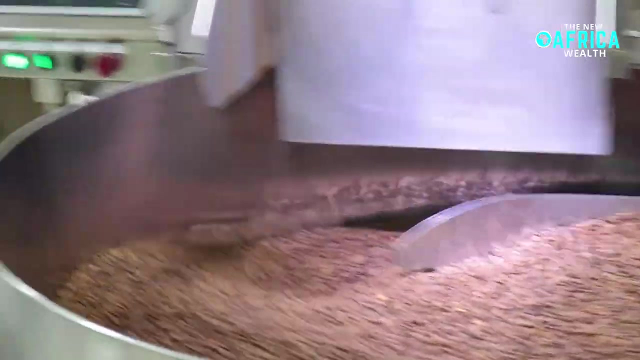 interested in starting a coffee roasting business is the initial cost. Coffee roasting equipment can be quite expensive, with prices often ranging from eighty thousand dollars and upwards for professional level roasters. On average, a small to medium-sized coffee roasting business can generate annual revenues ranging from one hundred thousand dollars. 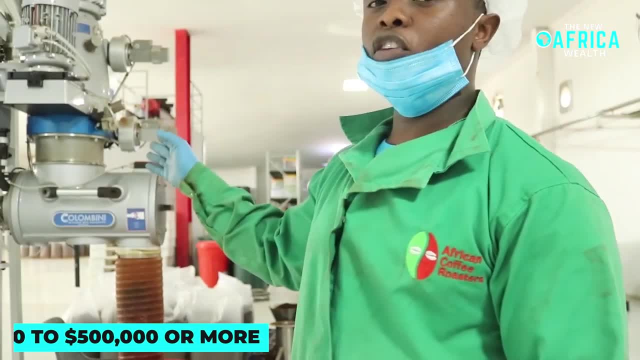 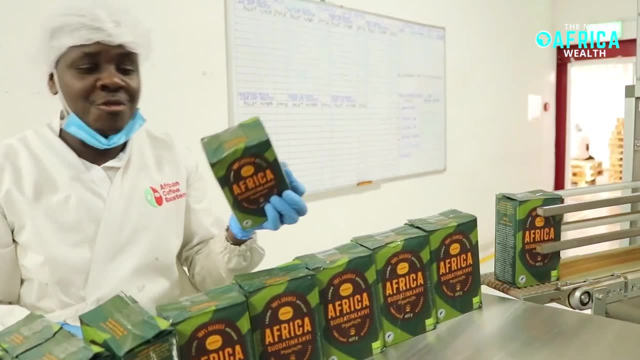 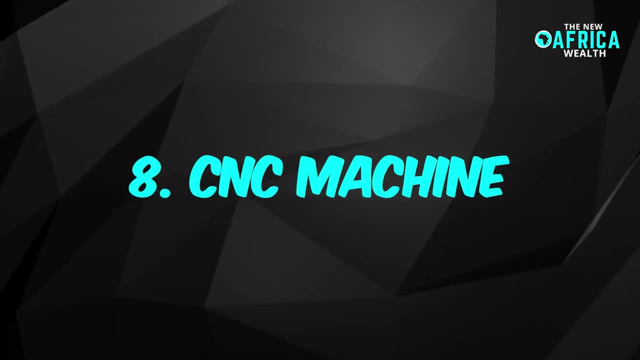 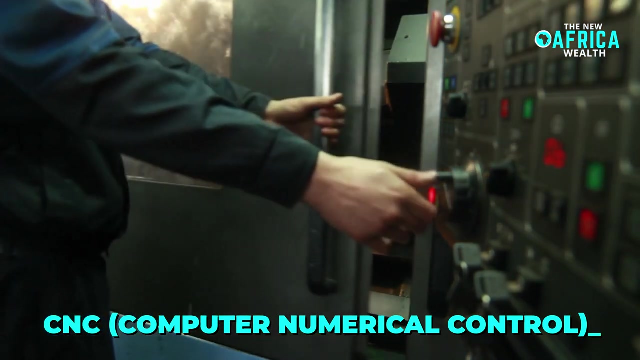 to five hundred thousand dollars or more. Some successful coffee roasters have reported annual revenues exceeding a million dollars, especially if they have expanded their operations and have a strong presence in the market. A CNC or Computer Numerical Control Machine is undoubtedly one of the most versatile and 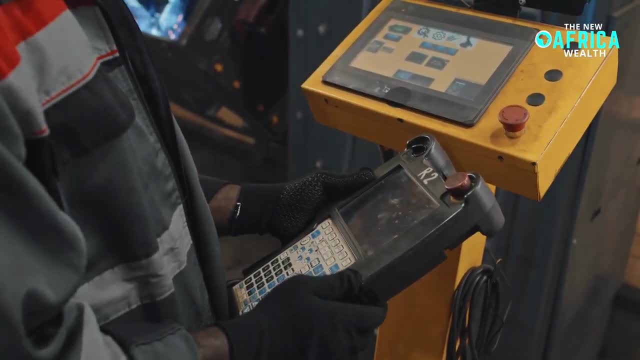 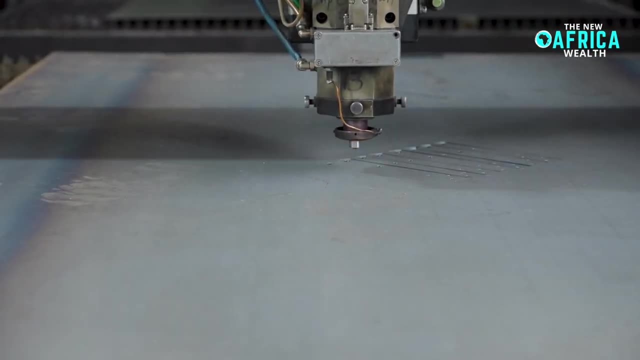 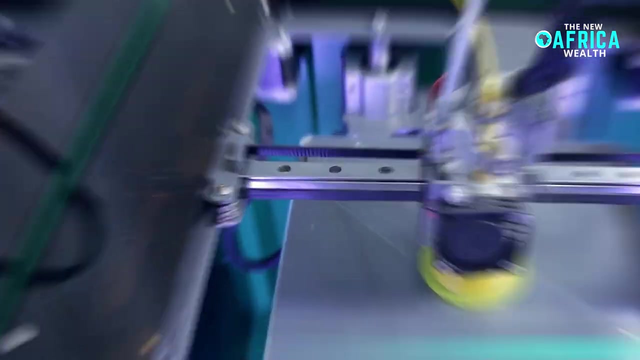 revolutionary tools in modern manufacturing and fabrication. Its ability to transform digital designs into precise physical objects with exceptional accuracy and efficiency has revolutionized various industries, From woodworking to metalworking, 3D printing to prototyping. a CNC machine empowers creators and entrepreneurs to bring their 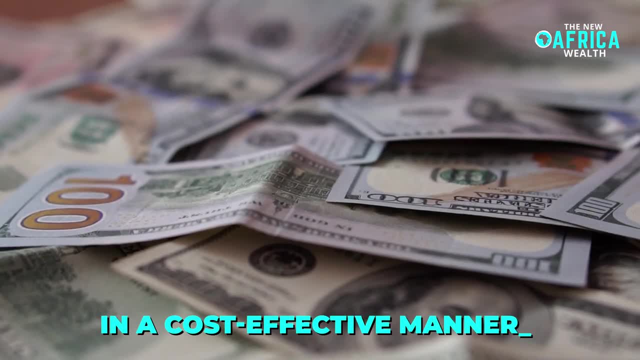 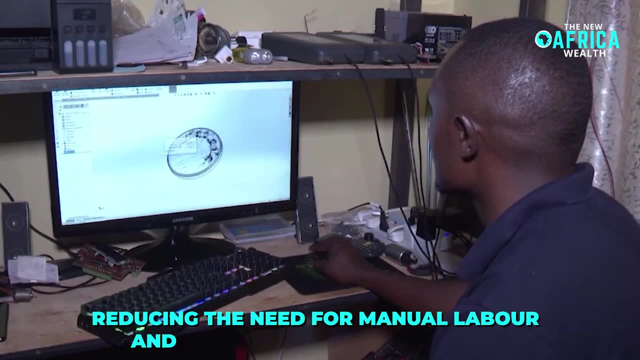 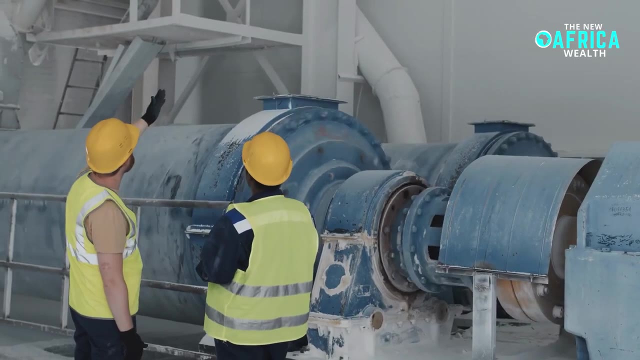 creative visions to life in a cost-effective manner. The beauty of a CNC machine lies in its ability to automate the manufacturing process, reducing the need for manual labor and increasing productivity. Once the initial investment in the CNC machine is made, the ongoing expenses primarily involve mills, drills, energy and raw materials. 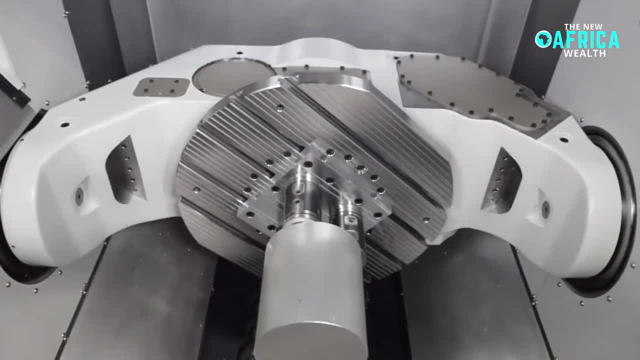 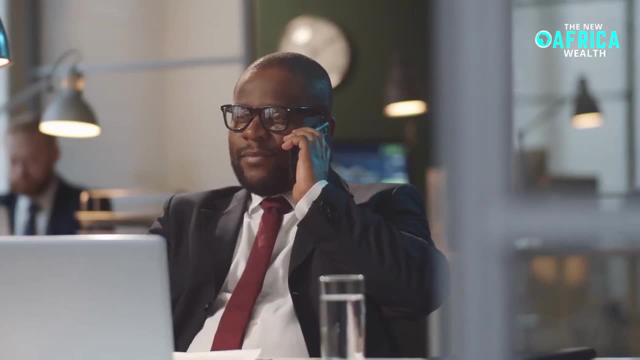 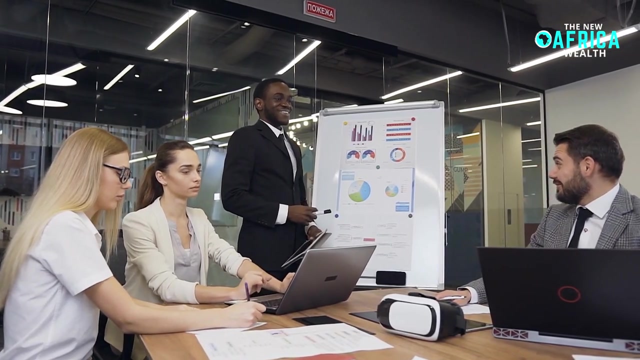 These consumables are relatively affordable and can be easily sourced, allowing businesses to control production costs and maximize their profit margins. Businesses can generate annual revenues ranging from tens of thousands to millions of dollars, depending on the scale of operations and the market demand for their products. 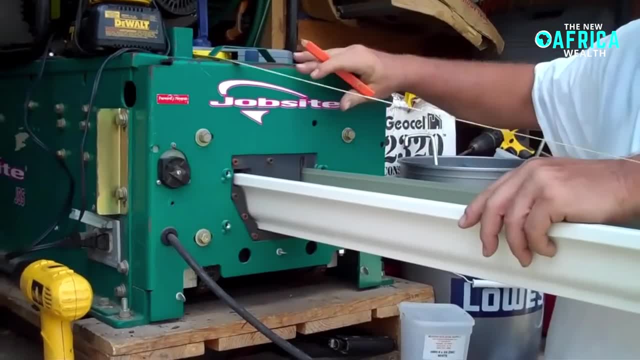 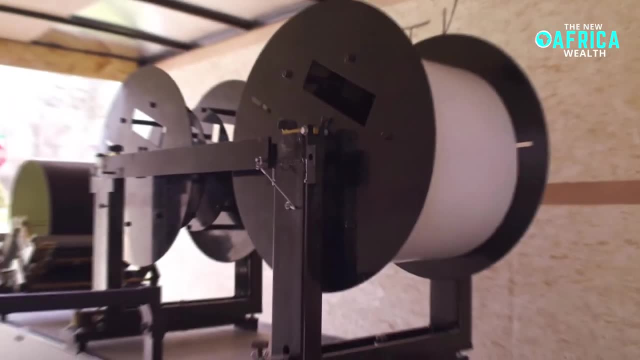 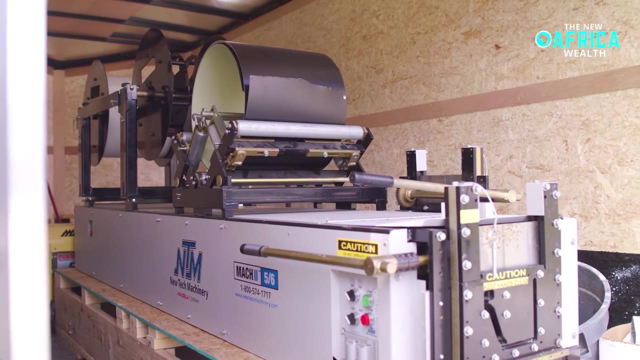 Gutter machines have proven to be fantastic investments, particularly for professionals in the construction and roofing industries, as well as other businesses involved in various crafts. These machines are specifically designed to fabricate seamless gutters, which are in high demand due to their enhanced functionality and aesthetic appeal. 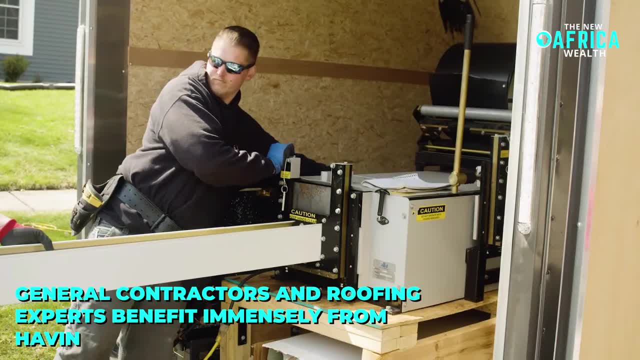 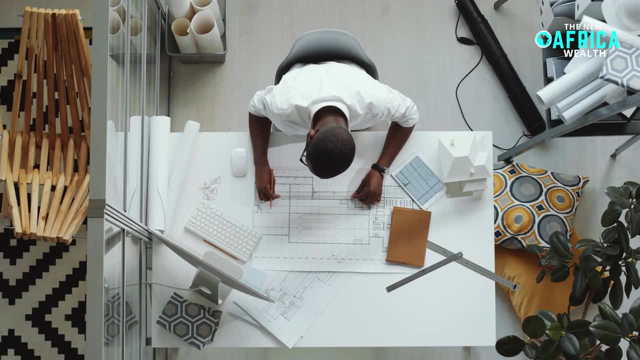 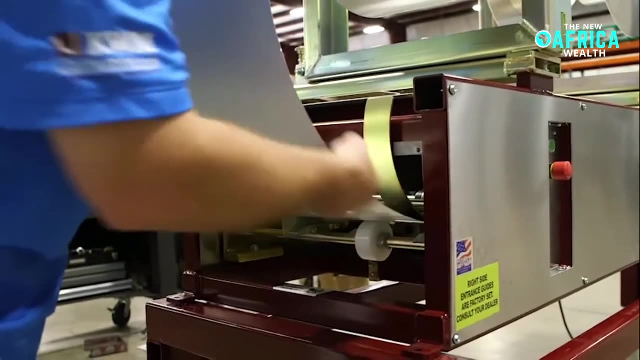 General contractors and roofing experts benefit immensely from having their gutter machines, as it allows them to customize gutters to fit specific building dimensions, reducing wastage and increasing overall efficiency. Moreover, businesses involved in exterior home improvement and maintenance can expand their service offerings by providing: 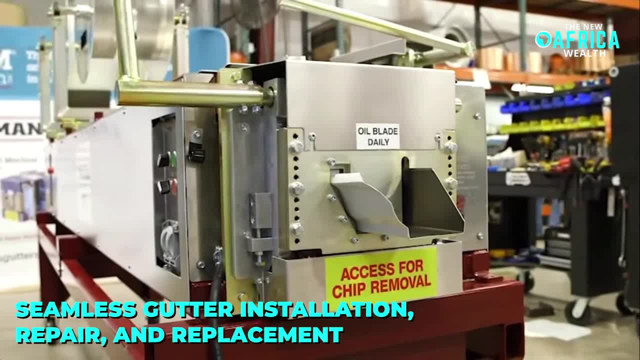 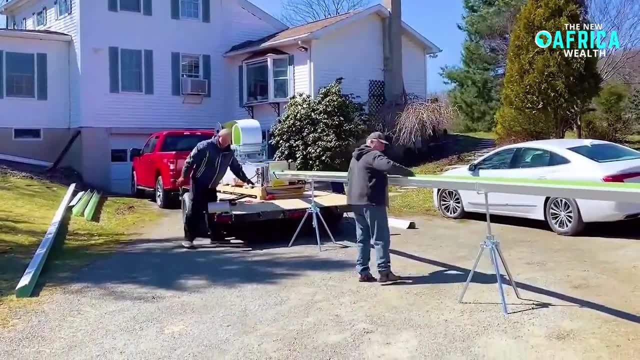 seamless gutter installation. Gutter machines can be used to repair and replace a building, thereby attracting more clients and enhancing their reputation in the industry. To make the most out of a gutter machine investment, it is crucial to fully understand the equipment's operation, care and maintenance. 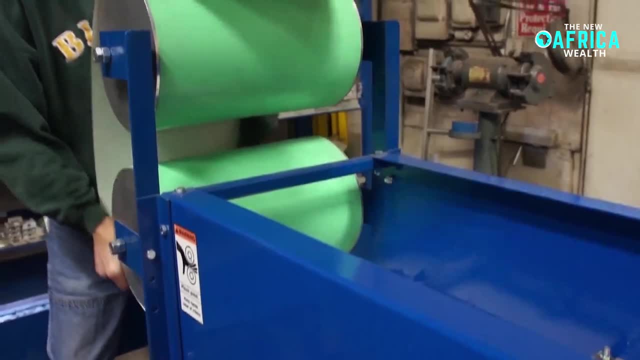 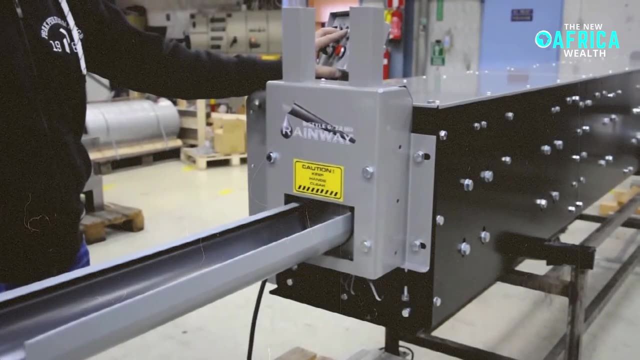 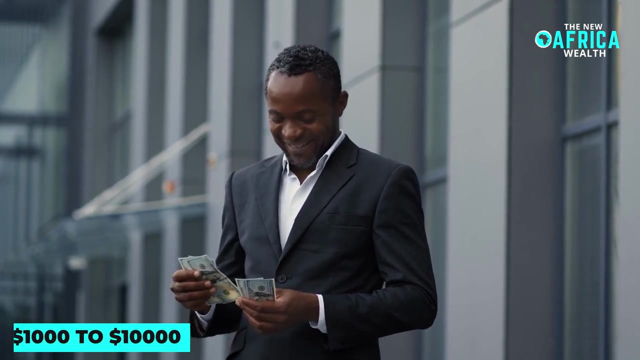 Regular upkeep and timely repairs can ensure the machine operates optimally, reducing downtime and maximizing productivity. Annual earnings from owning a gutter machine can vary. Smaller businesses may earn between $1,000 to $2,000.. While larger companies with more installations could make up to $100,000 per year. 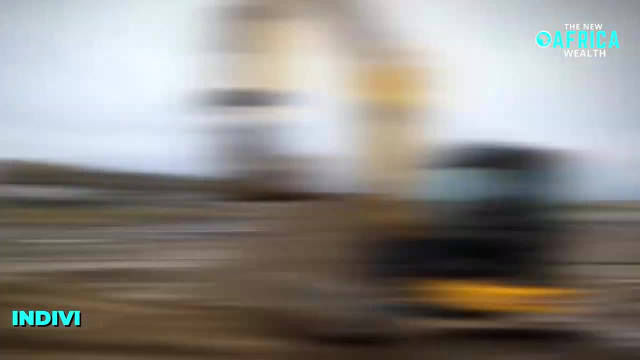 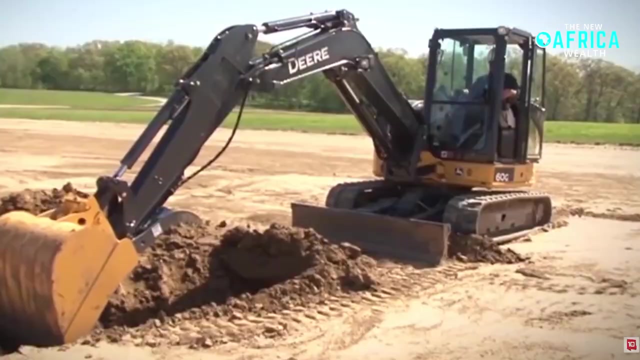 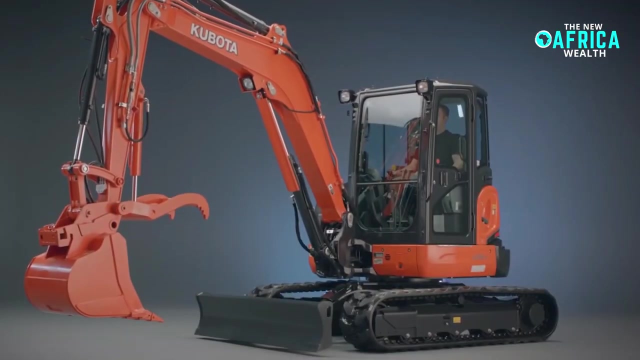 The MINI excavator is a highly lucrative investment for individuals or businesses in construction, landscaping or property maintenance. Its compact size and versatility make it ideal for executing various tasks, From digging trenches to landscaping and more. Many homeowners are attracted to this equipment for do-it-yourself projects and property improvements. 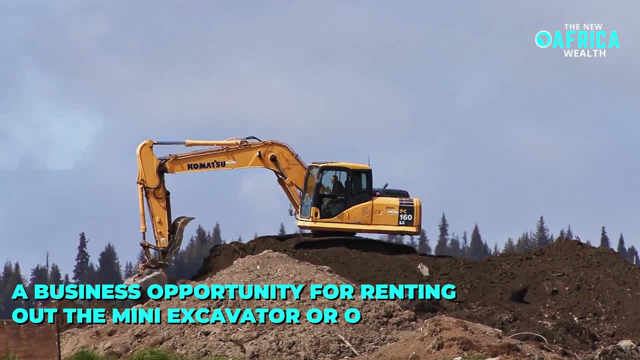 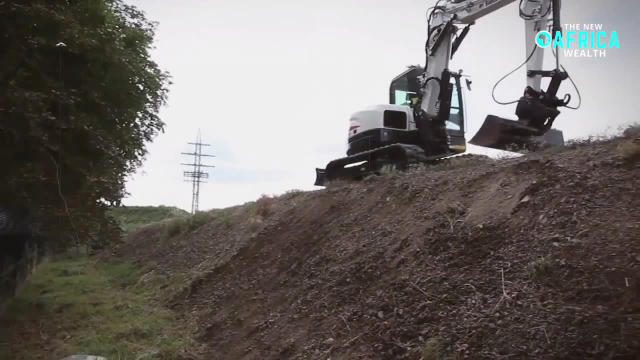 presenting a business opportunity for renting out the mini-excavator or offering services directly to homeowners. Annual potential earnings from renting or providing services with a mini-excavator could be up to $50,000, depending on the number of projects and demand in the local market. 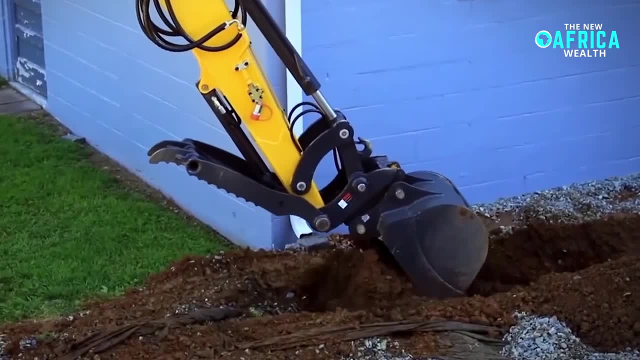 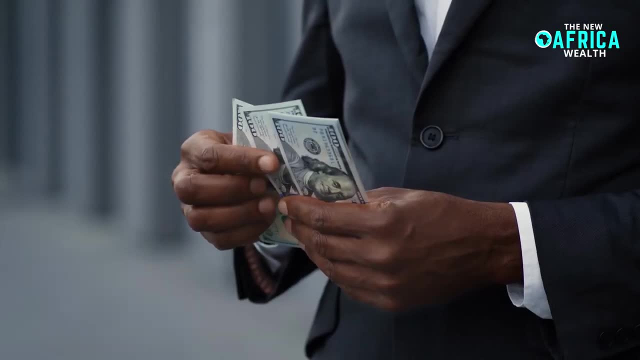 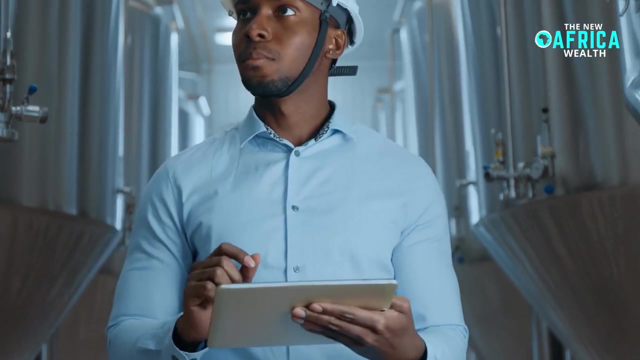 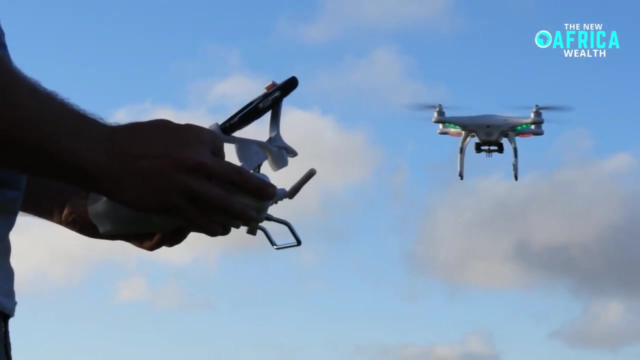 It offers a remarkable return on investment due to its efficiency and ability to handle diverse projects effectively, making it a valuable asset for generating profits and expanding business opportunities in the construction and home improvement sector. Drones have become not only enjoyable to fly, but also highly profitable tools with diverse commercial applications. 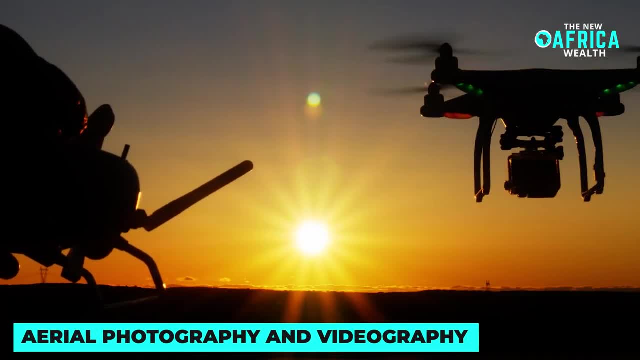 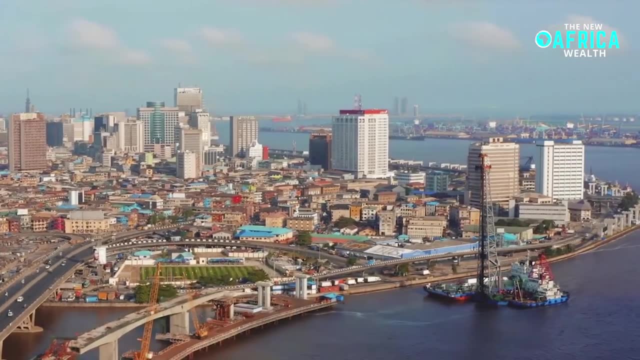 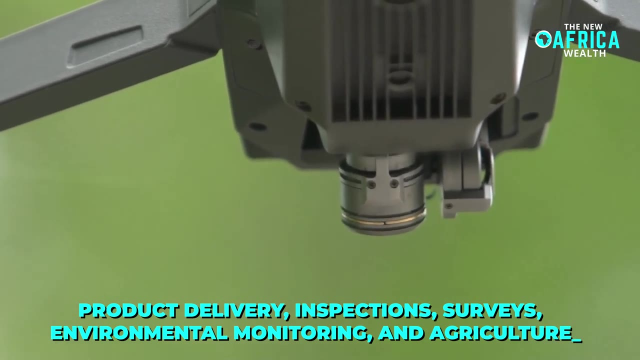 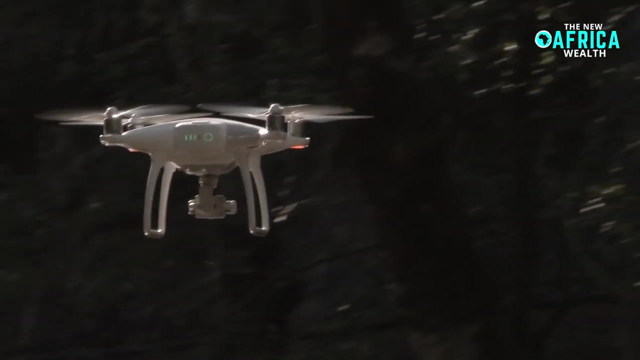 They are extensively used for aerial photography and videography, providing stunning shots for real estate, marketing, tourism and filmmaking industries. Additionally, drones are increasingly employed in product delivery inspections, surveys, environmental monitoring and agriculture. Their ability to access hard-to-reach or hazardous locations makes them invaluable for various industries, enhancing safety and efficiency. 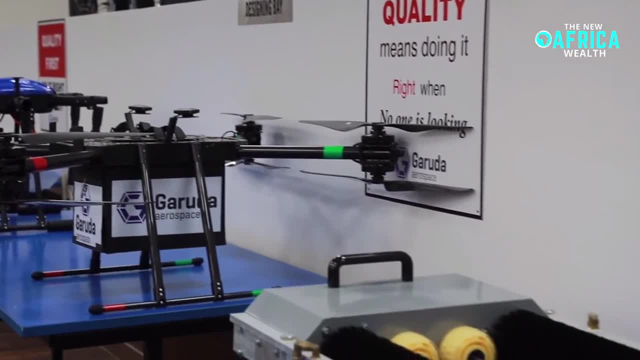 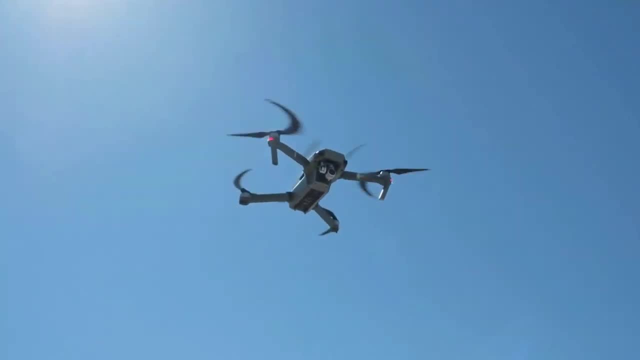 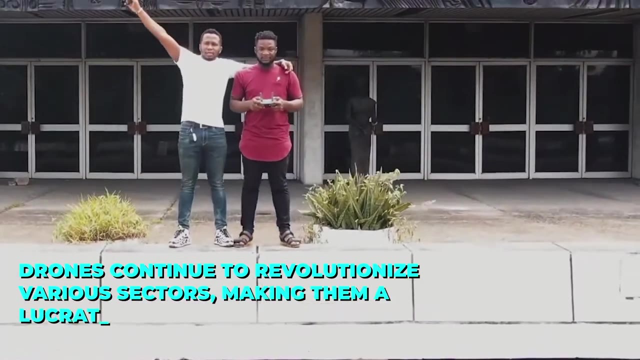 Entering the drone service industry offers a wide range of services and it offers entrepreneurs significant earning potential, where investors to make $100,000 and more annually, depending on the range and complexity of services provided. With their versatility and expanding applications, drones continue to revolutionize various sectors. 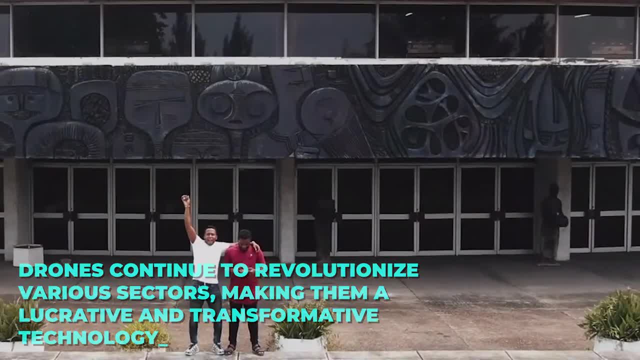 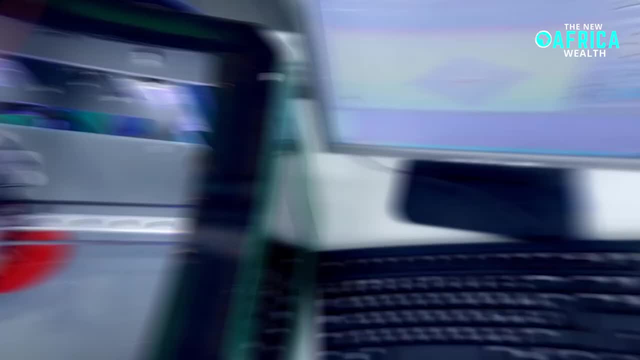 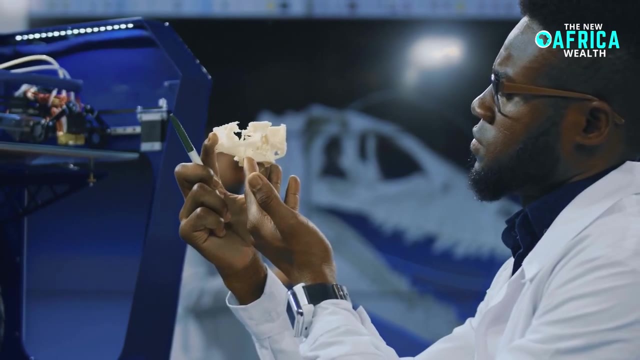 making them a lucrative and transformative technology. 3D printers offer a wealth of opportunities for creative, smart and innovative technology. 3D printers offer a wealth of opportunities for creative, smart and innovative technology. Constructing 3D printers costs, to monetize their skills and imagination, between 17 and 18 hundred dollars. 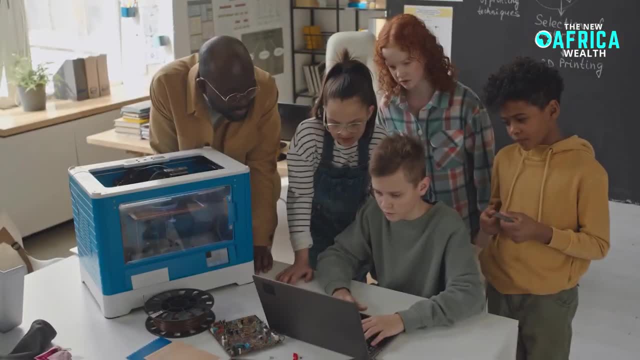 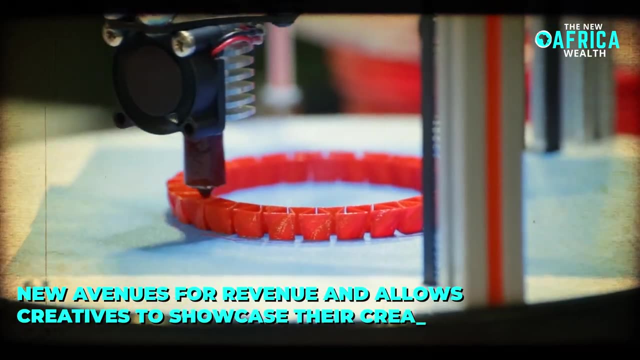 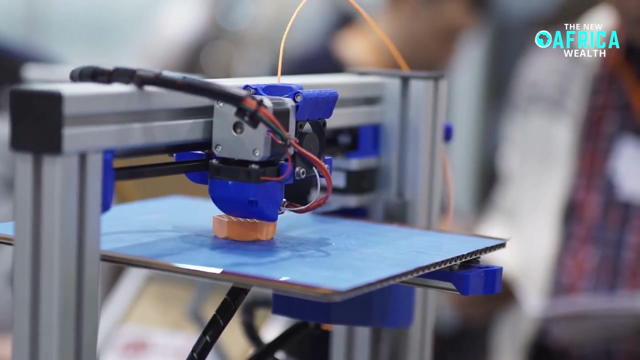 Artists and designers can create and sell unique 3d printed goods, catering to niche markets and offering personalized products. These opens up new avenues for revenue and allows creatives to showcase their creativity and craftsmanship. Additionally, providing 3d printing services to businesses and individuals offers a steady income stream. 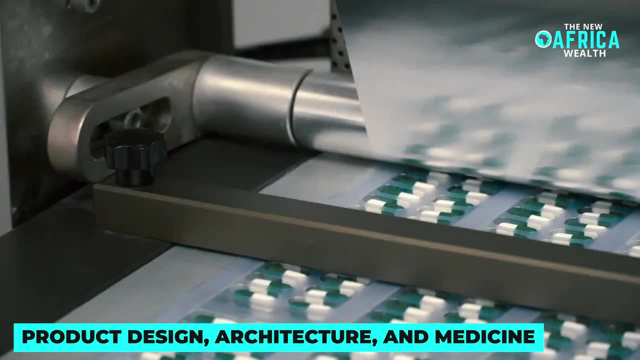 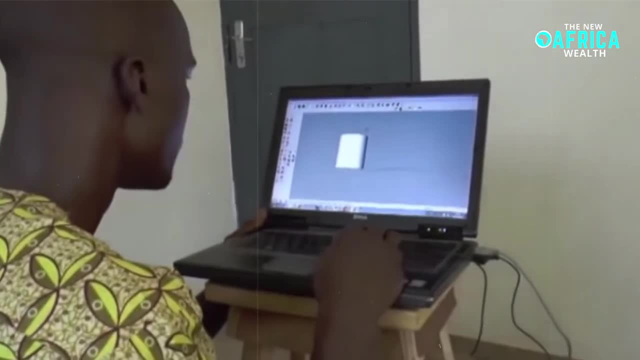 Industries like product design, architecture and medicine increasingly rely on 3D printers. Industries like product design, architecture and medicine increasingly rely 3D printers 3D printing for prototyping and production, creating a demand for professional 3D printing. 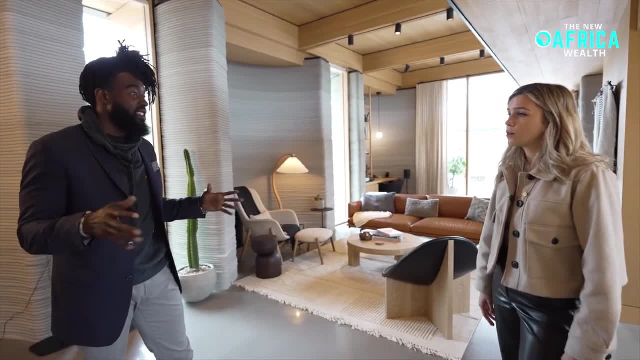 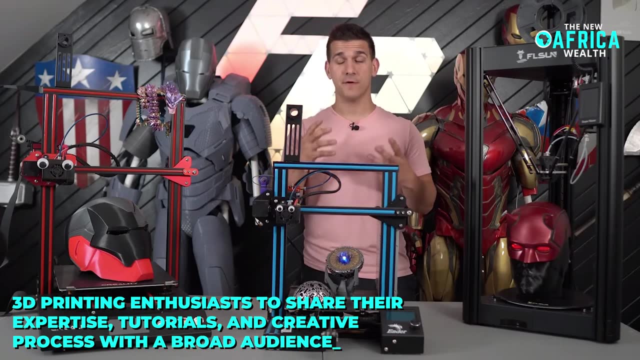 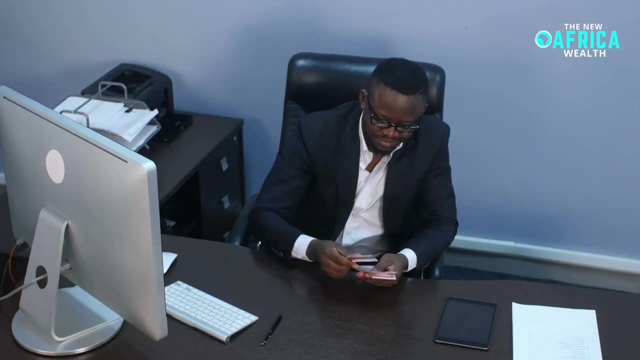 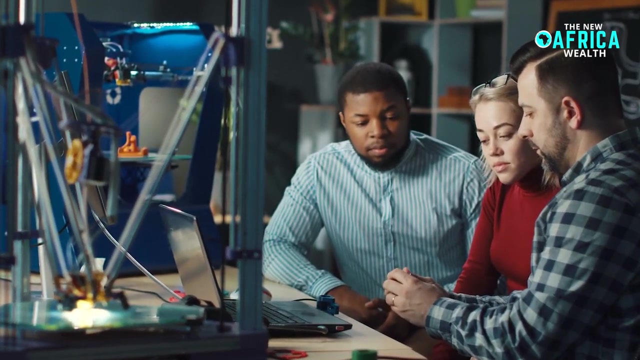 services. Moreover, content creation through YouTube channels allows 3D printing enthusiasts to share their expertise, tutorials and creative process with a broad audience. This not only inspires others, but also presents an opportunity to generate income through advertisements and sponsorships. With 3D printing's versatility and growing popularity, creatives have a world of possibilities. 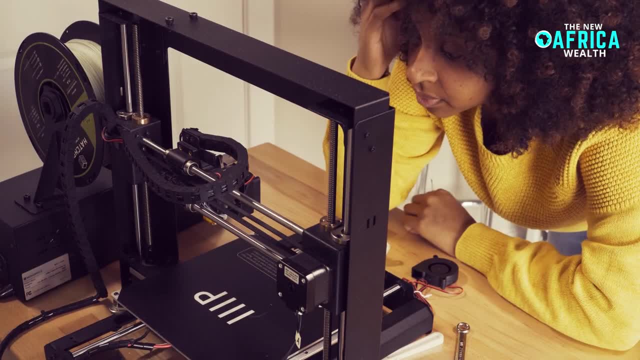 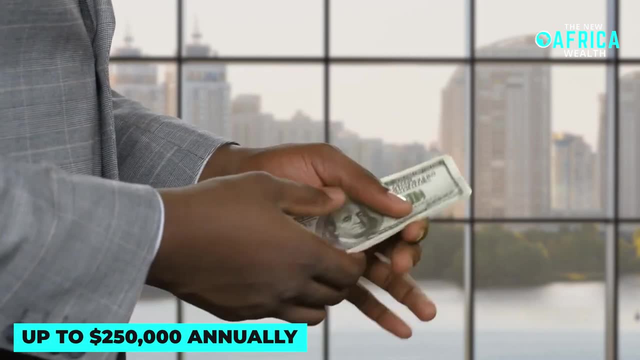 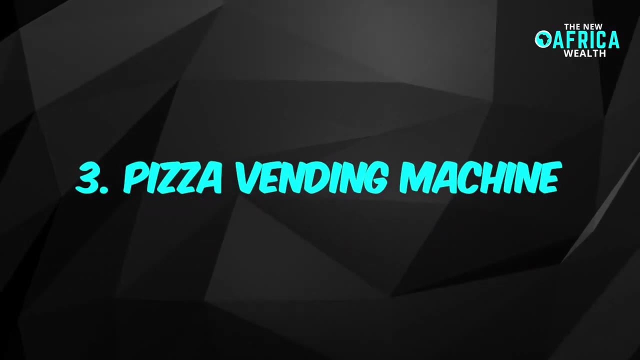 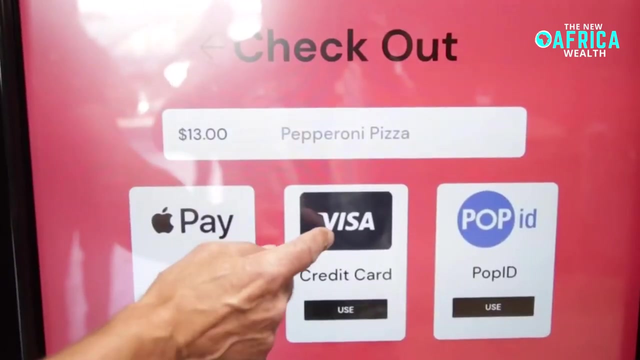 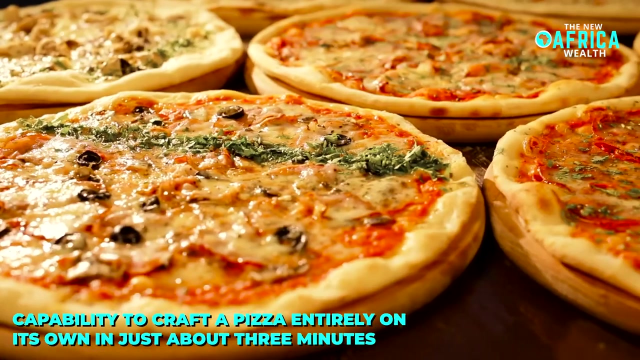 at their fingertips, enabling them to thrive in the dynamic landscape of 3D printing and digital creativity. Potential earnings could be up to $250,000 annually. The pizza vending machine represents a remarkable innovation in the world of food service and marketing, With the capability to craft a pizza entirely on its own in just about three minutes. these 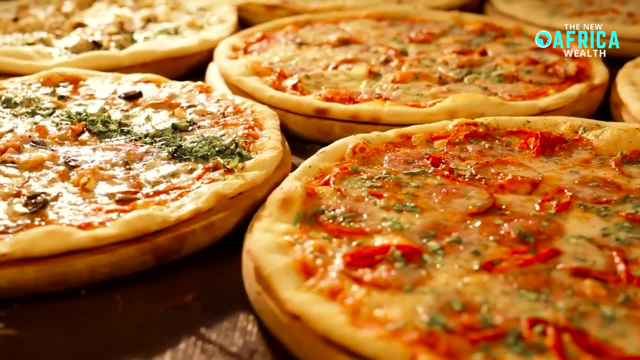 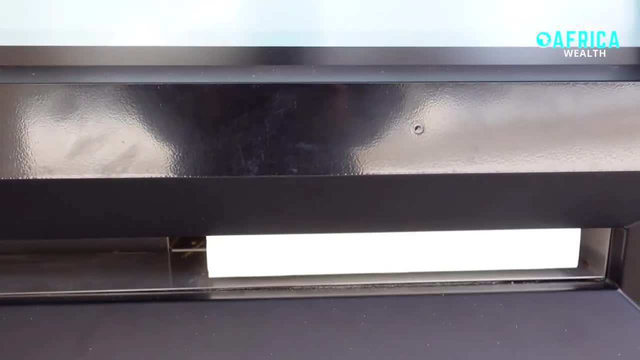 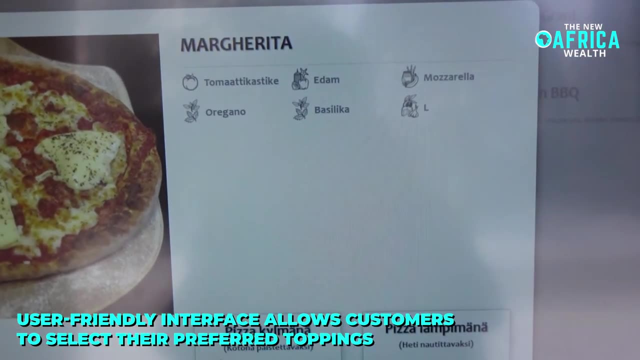 machines are reshaping the way people satisfy their cravings for a quick and delicious slice of pizza. Installed at any vantage point, these machines provide convenient access to freshly made pizzas around the clock. The user-friendly interface allows customers to select their preferred toppings and watch. 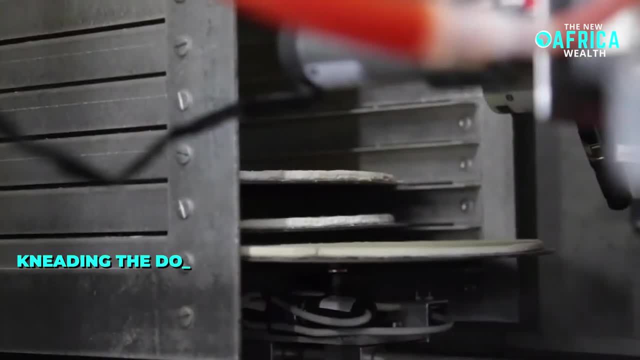 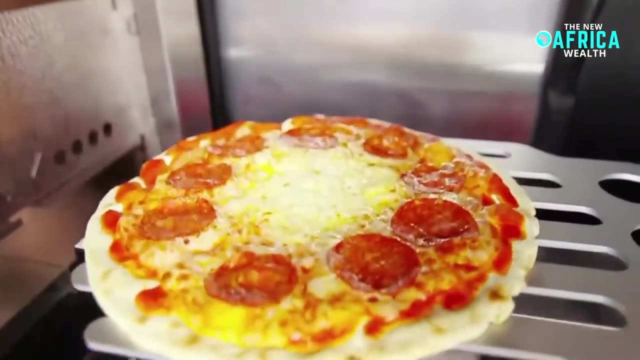 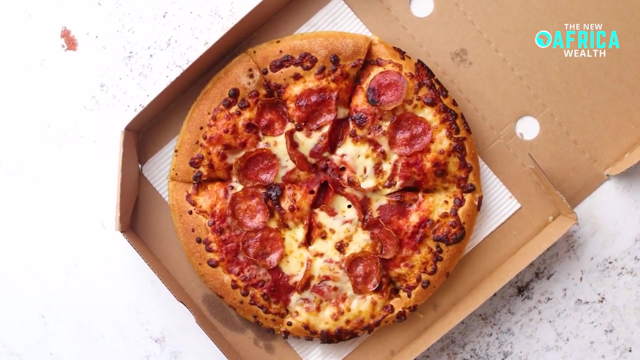 in awe as the machine springs into action, kneading the dough, spreading the sauce and layering on the toppings with precision and efficiency. The enticing aroma of freshly baked pizza wafts through the air, drawing in hungry patrons, and within minutes they are rewarded with a piping hot and perfectly cooked pizza ready. 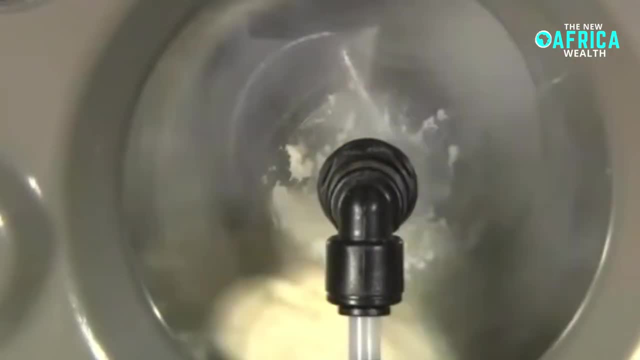 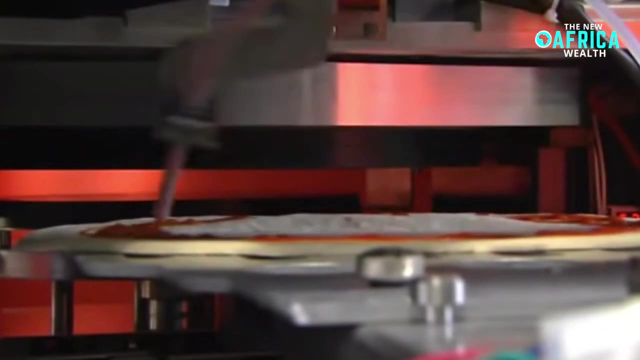 to be savored. One of the most appealing aspects of the pizza vending machine lies in its economical operation. The machines are designed to minimize waste, ensuring that only the necessary ingredients are used for each pizza. This not only reduces food costs, but also can help save money. 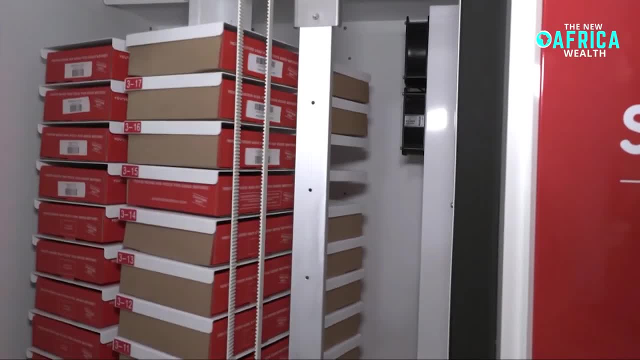 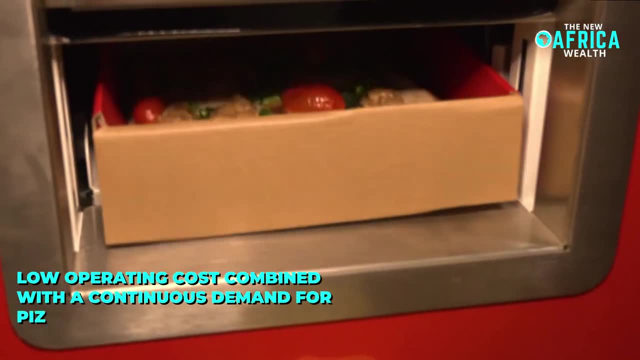 The machine is designed to minimize waste, ensuring that only the necessary ingredients are used for each pizza. The machine also contributes to sustainability and environmentally friendly practices. Moreover, the low operating cost, combined with the continuous demand for pizza, makes these machines highly profitable investments. Past performances of pizza vending machines have demonstrated an extraordinary average return on investment, making them a lucrative option for entrepreneurs seeking to capitalize on the fast-food market's growing demand. Potential earnings are using up to $100,000 or more. The pizza vending machine is designed to minimize waste, ensuring that only the necessary ingredients. 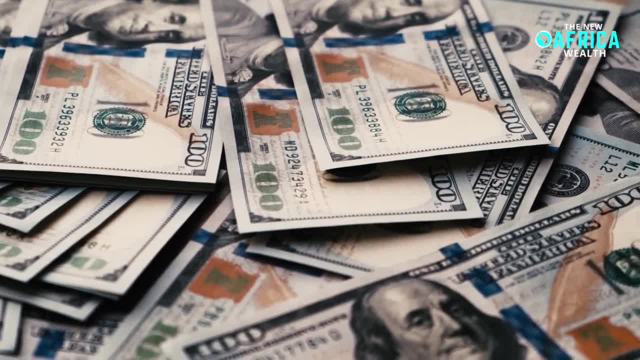 are used for each pizza. With 100% software and computer software, you can lease-free on the consumer's emulate years of customer interest and let your abbreviations and customers use it once they 've aren't satisfied with their retail hits fromGERMA. 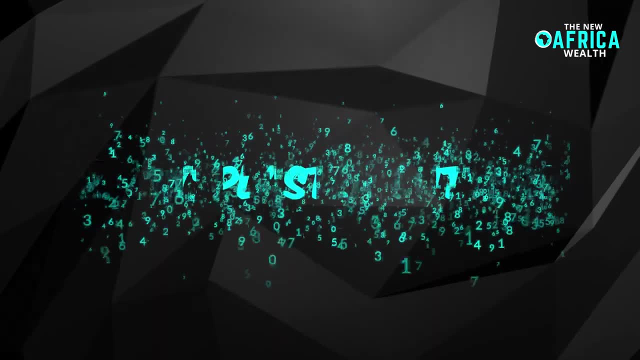 Creating proper, sustainable prices with their unique equipment. in very simple우, You can create your own сеin, which measures to create even more value for people's income. and when you're maybe thinking of something small, you've got to think of your quite. You can get from times to times by씩, using their unlimited cost, which saves money, or through different tools, including your own resume, e- muscles, etc. At the same time, you don't have to cost as much as somebody as you may want. 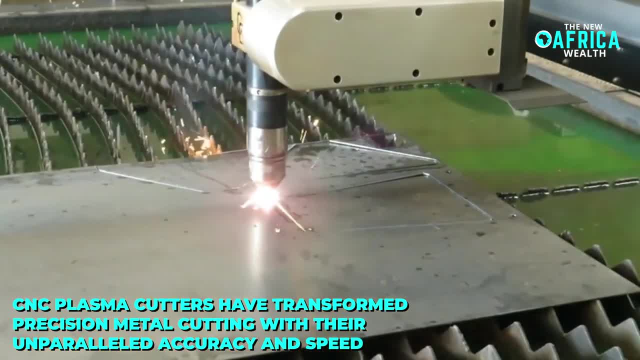 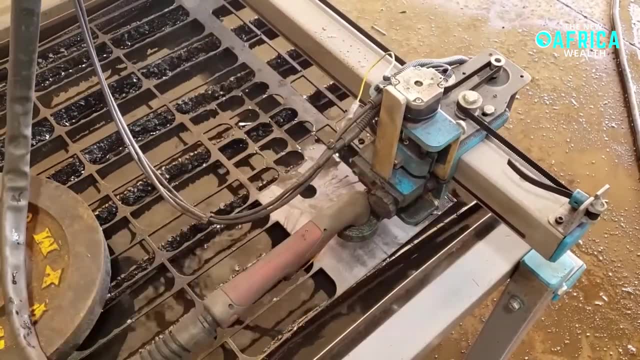 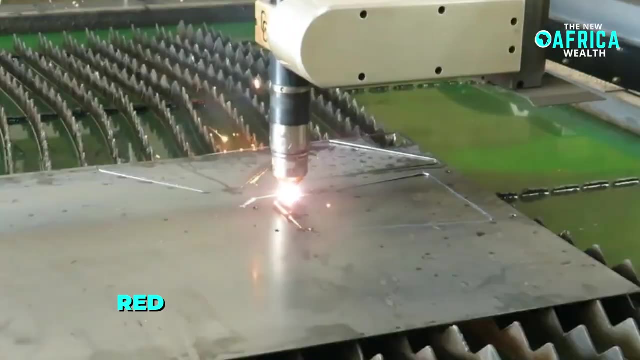 They've already been on the roof of your orders for a year, though, and those orders tend to continue to go up and down For more than recordings or references on low- streamlined 에�ین, aluminum and stainless steel. The automated process ensures consistent results, reduces production time and minimizes material. 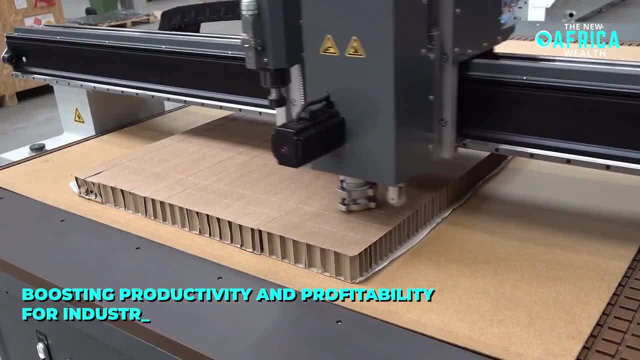 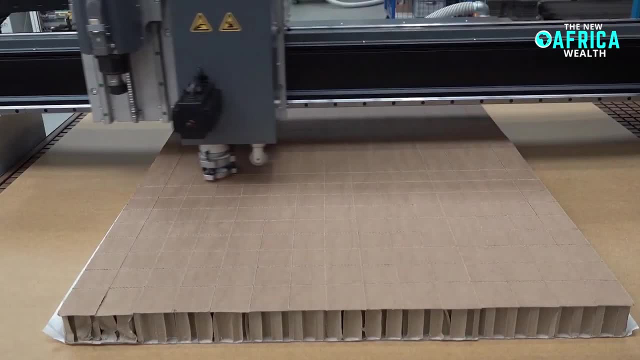 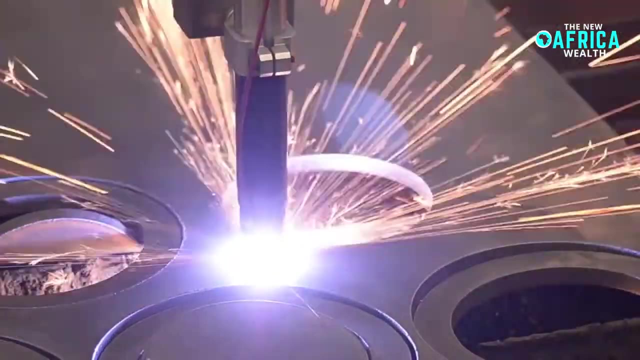 wastage, boosting productivity and profitability for industries like manufacturing, automotive, aerospace and art. CNC plaster cutters could provide entrepreneurs with up to $50,000 or more, depending on the location and availability of jobs. The versatility of CNC plasma cutters makes them a valuable tool for both heavy-duty industrial. 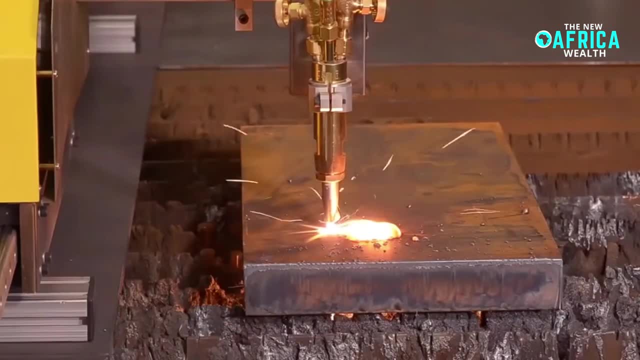 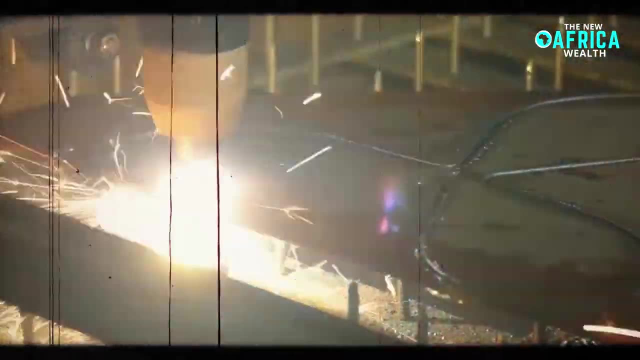 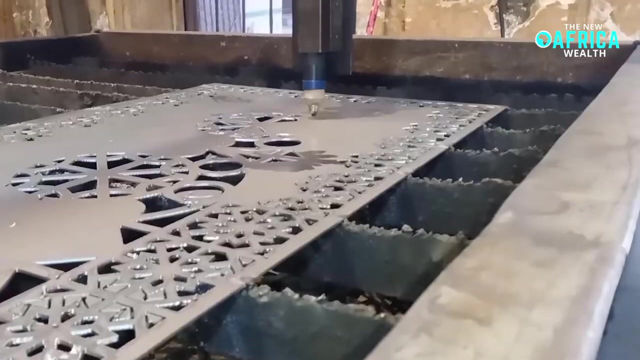 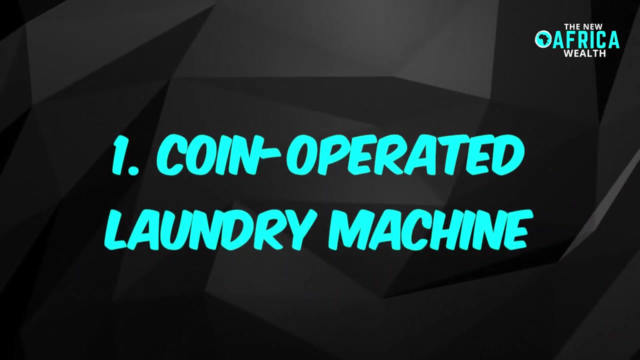 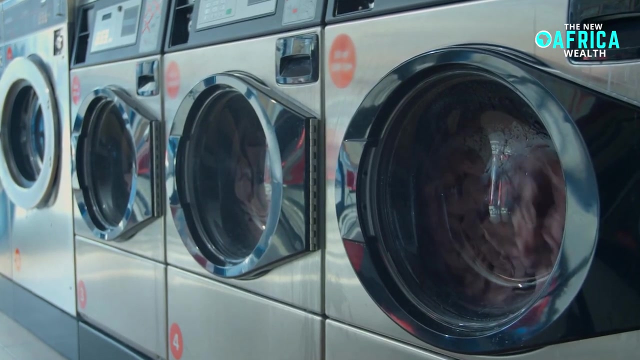 projects and artistic creations, providing endless possibilities and new employment prospects in the metalworking sectors. With their ability to revolutionize precision metal cutting, CNC plasma cutters are paving the way for increased efficiency and innovation in various industries. The concept behind coin-operated laundry machines is straightforward and user-friendly.